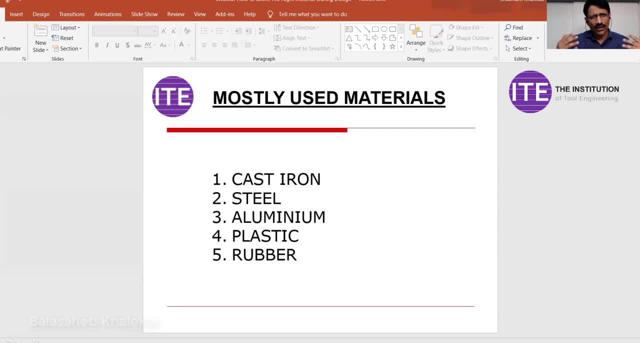 machinery, or oil and natural gas, whatever is field or piping industry. These five materials you are going to deal with Understand the example of a car: Body components. the material is steel. Dashboard instrument panel. the material is plastic. Piston, clutch housing. 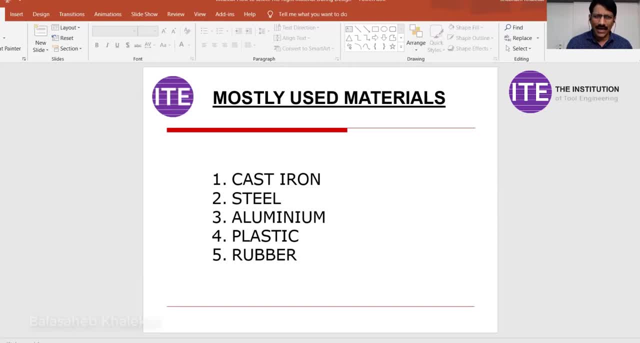 gearbox housing: the material is aluminium. Tyres, floor mat trim area: the material is rubber. So this is how we have to understand and, in this particular, if we consider all these five materials, what you have to study right from density. So these points we are going to understand. 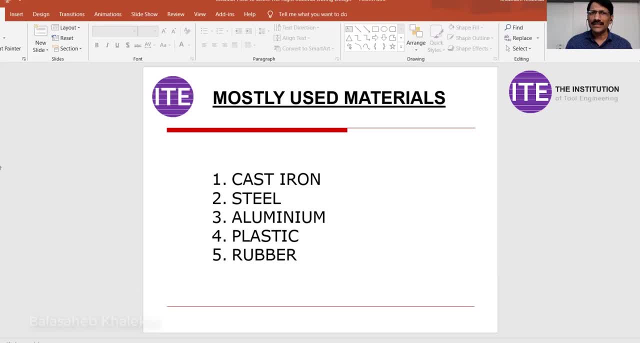 the advantages and limitations also and the, we can say, the properties. So the first material is cast iron and this is one important question generally asked during interview. All the contents, cast iron contents, those the main elements in cast iron: iron, carbon, silicon, manganese, sulfur and phosphorous. this is the contents. 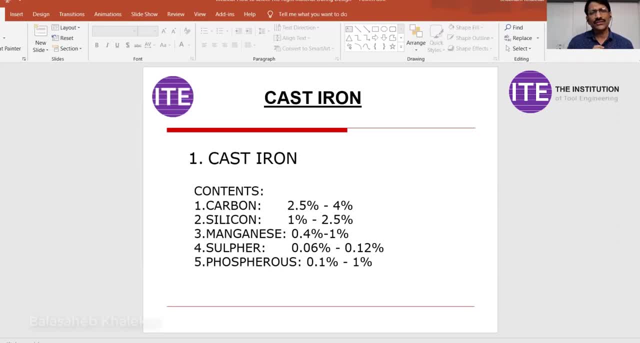 So general value you must know, and carbon percentage is very, very important. At least you should know the carbon percentage and even though some sometimes it is not possible to remember all the values, but at least content you should know, That is, silicon, manganese, sulfur and phosphorous. 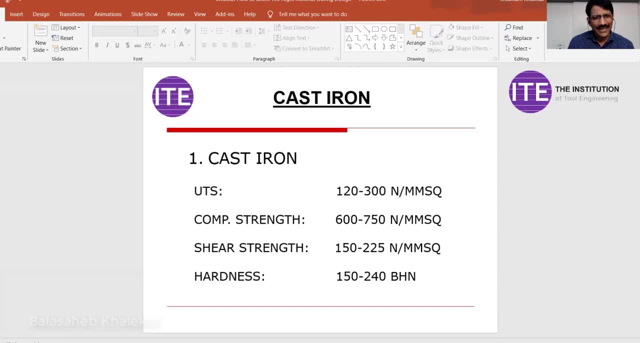 Then the various we can say strengths. ultimate tensile strength: this is the range compressive strength. then compressive strength in case of cast iron is higher than steel. that we have to understand. Then hardness: it is in BHN Brinell Hardness Number. 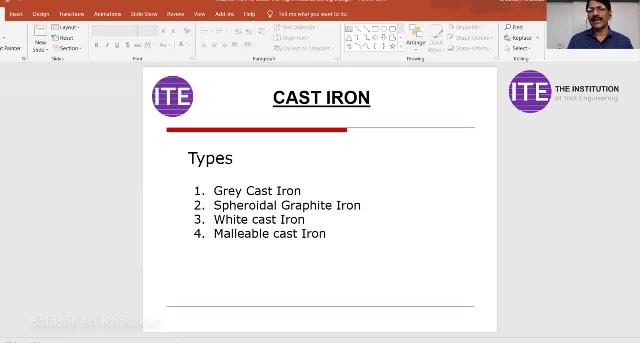 Types of cast iron. gray cast iron is the most popular material, Then spheroidal graphite iron. spheroidal graphite iron is having property in between steel and cast iron. Steel is having high tensile strength. Cast iron is having high compressive strength. 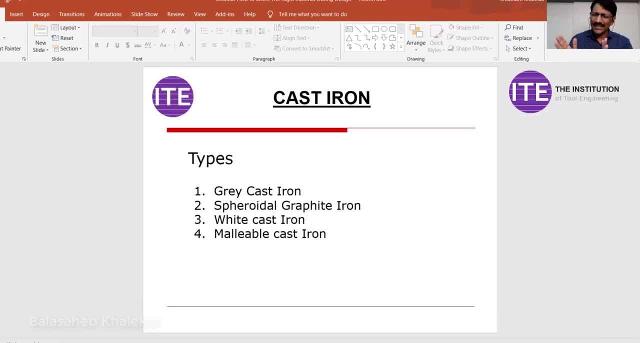 So in between, Sg iron is having more tensile strength than cast iron. Steel is having poor castability property. Cast iron is having excellent castability property, So Sg iron is having better castability property than steel. So Sg iron 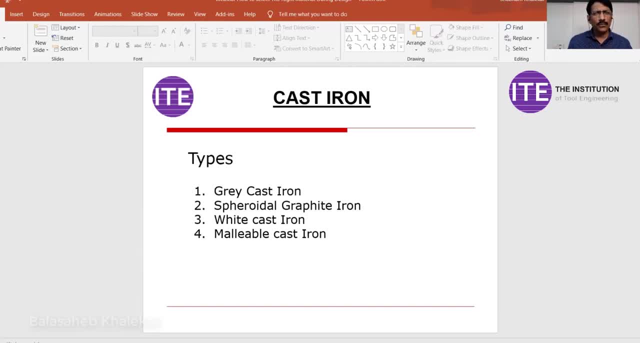 is also called as a nodular cast iron and all components. you can see where there is a vibration or shock loads are there, and when the complex geometry is there, then you have to go for sg iron material. so steering components, axle components, all components, the material is 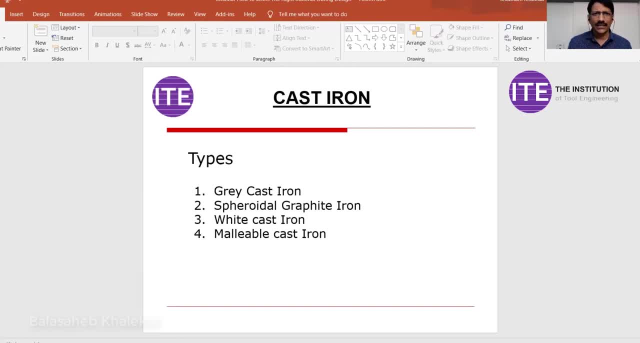 sg iron and gray cast iron: engine block, engine head, gearbox housing all such components. they are made up of gray cast iron, then white cast iron and malleable cast iron. these are the main types of cast iron. if you understand the advantages of cast iron- low cost, excellent. 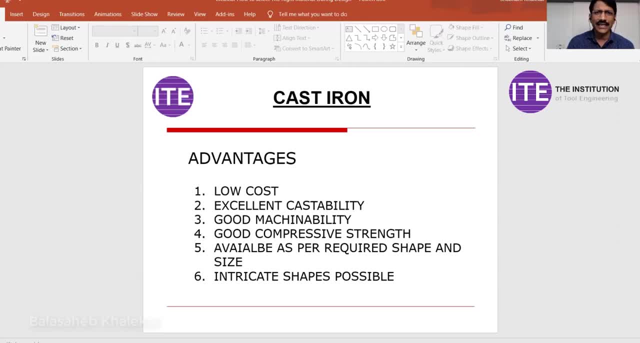 cast ability property means you can take or produce any critical shape. good machinability and here one important thing, have you observed- machining of cast iron and steel. so when you are machining cast iron generally, you will find that no coolant is required because the graphite in this particular material it is in the free form. 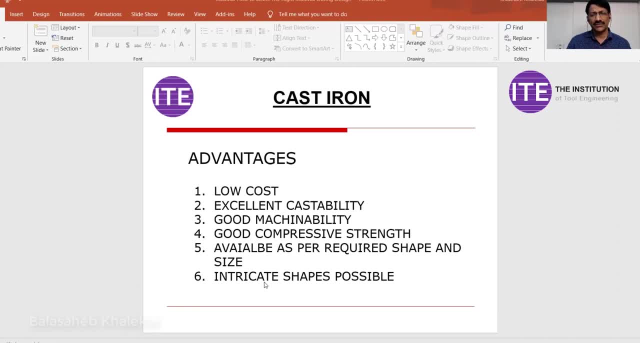 so that acts as a coolant. the next point is good compressive strength, then available as per the required shape and size. very important point. see, when you are completing your project work or your drawing is ready. you have to understand the other area about the machining or manufacturing part as well, when you are in the design stage. 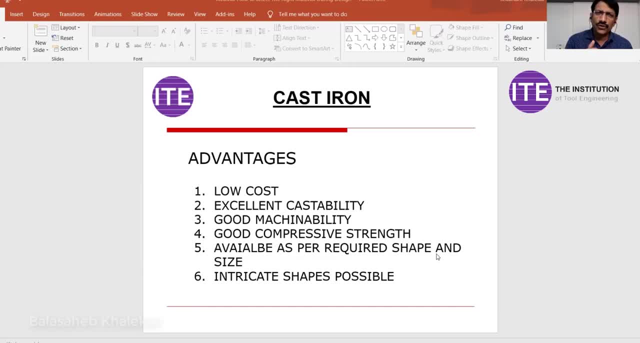 and when you have to understand how you are going to procure the material. so if it is a cast iron material, you can procure the material as per the desired shape and size, which is not, which is difficult, in generally, steel. in case of steel, you have to procure the material as per the availability. 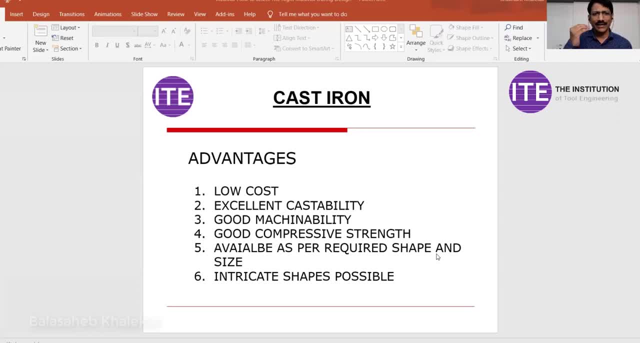 means whatever is the size available in the market and in case of cost, time, how this is possible. it is possible because you can go for a particular pattern that is made up of thermal cool and from that thermocool you can procure the casting as per the desired shape and 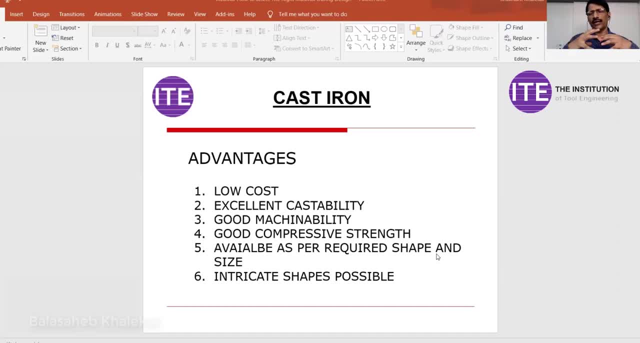 size. so here, in this case, what is the advantage? you are reducing the material, you are reducing your machine time and the cost. next point: intricate shapes possible. yes, when it is a class time, any critical shape can be produced. now let us understand the limitations of this particular material: cast time. it is a brittle material. careful handling is required, low finish. 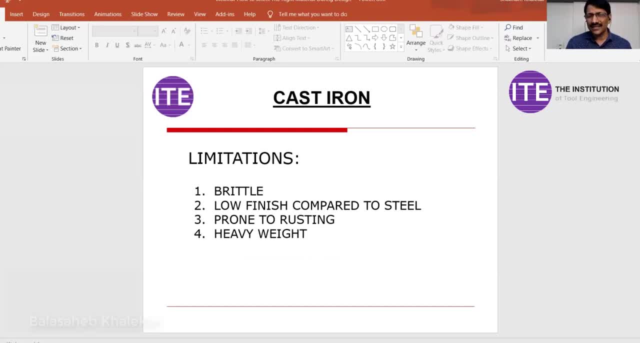 compared to steel. that we have to understand. then, prone to rusting: yes, possibility of rusting is there, and heavy weight. so in case of conventional methods, generally this is avoided. then applications, as we studied: engine block, engine head, gearbox housing, clutch housing, many applications. then coming to the next point, that is steel, and it's a vast difference. and one more important question: 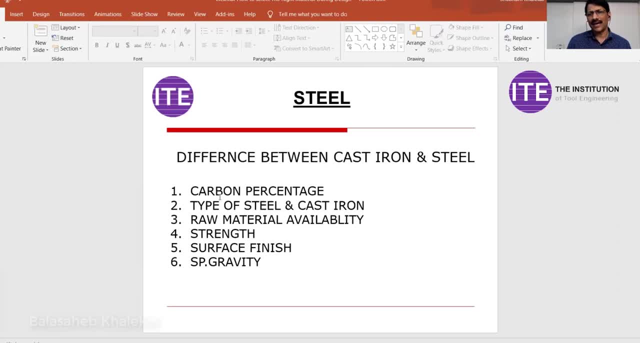 generally asked during interview: what is the difference between cost, time and steel? so these are the important we can say points. you have to answer which are those points? carbon percentage: so it may start with 0.03 up to 1.2 percent. so as per the carbon percentage, there are again types. 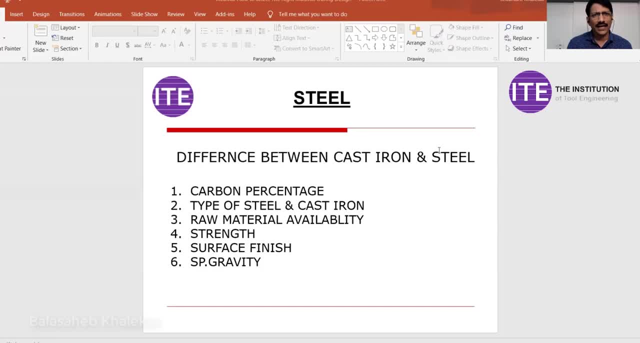 like low carbon steel, medium carbon steel and high carbon steel, so mild steel most commonly used in the industry. which are those areas right now that are used in the industry. which are those areas right from fastener, various back plates, support plates, fixture structure or we can say, fabrication. 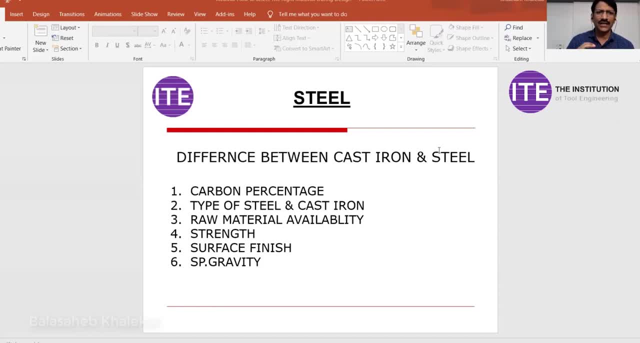 everywhere you can see mild steel, then the medium carbon steel. you have to understand that application. most of the forging components, the material, like flanges, we can say various shafts. the material is medium carbon steel and high carbon steel, whether it's a drill or reamer like that. then you have to understand about the 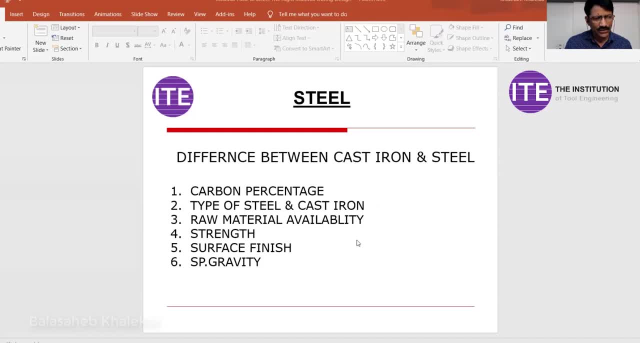 raw material availability. i told you raw material available. in case of cross time that is possible with any shape and size, which is not possible in case of steel. then strength: high strength in tensile strength in steel. high compressive strength in cross time. surface quality: better in steel. then cast time: it is lesser than this, then specific: 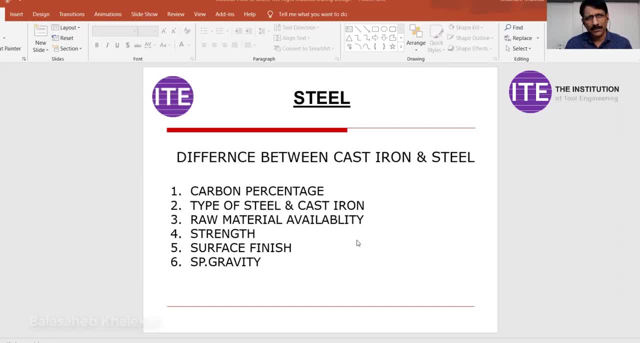 gravity. very small difference is there? seven point two gram per centimeter cube in case of cast time, 7.8 gram per centimeter cube in case of steel. Then types of steel. I told you about. it is a huge subject, friends, but what you have to focus mainly low carbon steel, medium carbon. 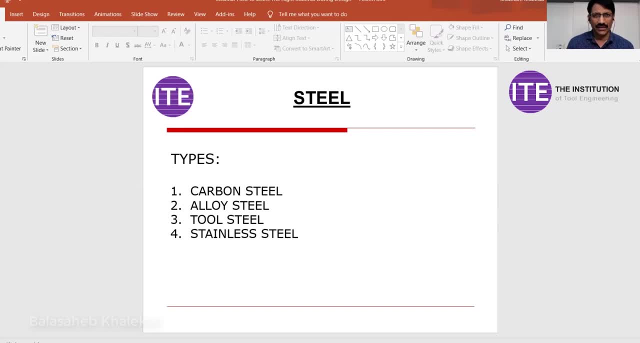 steel and high carbon steel, then alloy steel, Alloy steel, various again different types, tool steel and stainless steel. We can say these are the broad four categories, but the subject is very vast And what you have to understand again, what are those alloying elements and what? 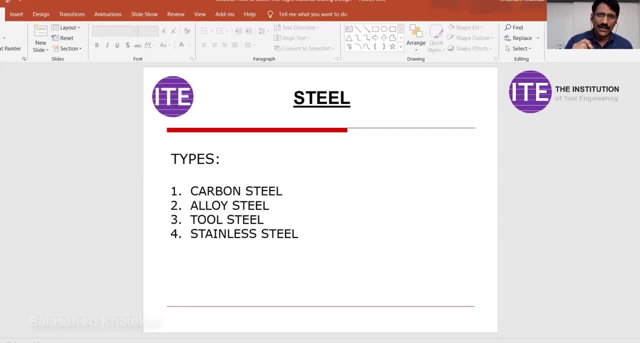 is the property you are going to achieve when you are adding a particular specific material, Then advantages: high strength, better accuracy, better surface finish and thin sections can be made compared to cross-stripe. that is possible. Again, limited number of materials, but the subject is very vast And what you have to understand. 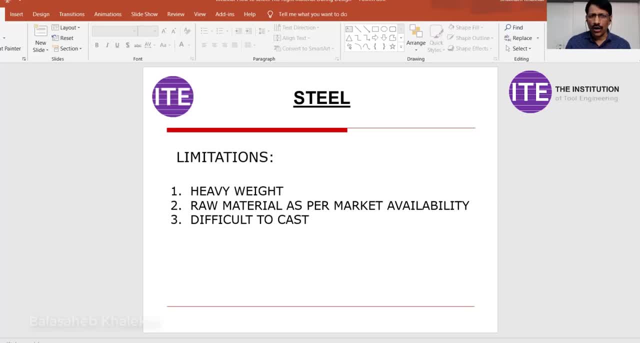 limitations: heavy weight raw material as per the market availability, and difficult to cast. Difficult to cast means casting of steel. Generally you will find problems of shrinkage. that is a defect. The next point is aluminum. Now you must have observed that most of the 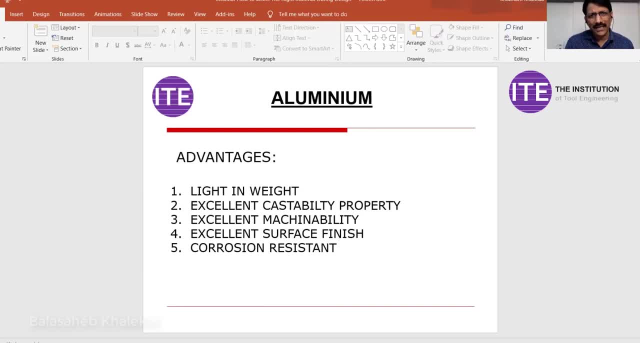 components are now being replaced from steel to aluminum. The main reason is weight, weight constraint. One more is that we can say it is not affected by other atmospheric conditions, and all That is one important thing. And advantages of aluminum: first of all, lighting, weight, Friends, three important materials. 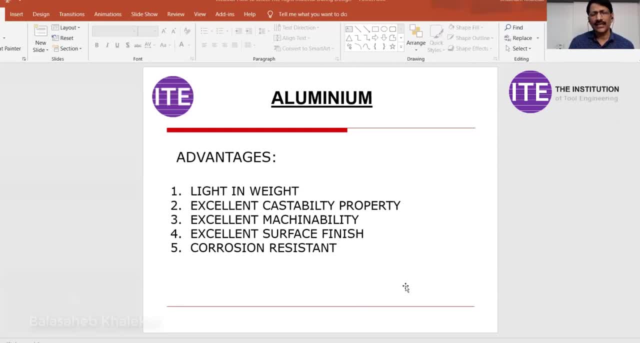 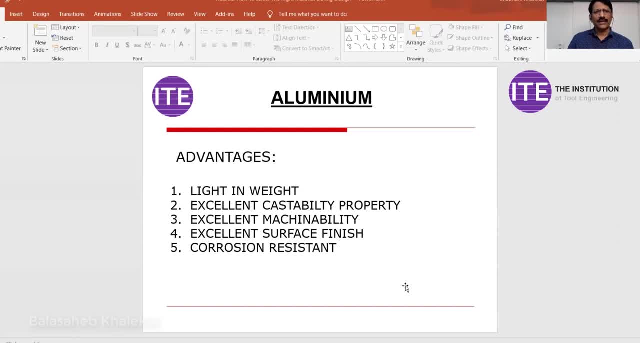 you. That is 7.8 gram per centimeter cube, So excellent castability property. It has very good castability property And that is the reason you can produce any critical shape in aluminum. Excellent machinability is there. Excellent surface finish is achieved.